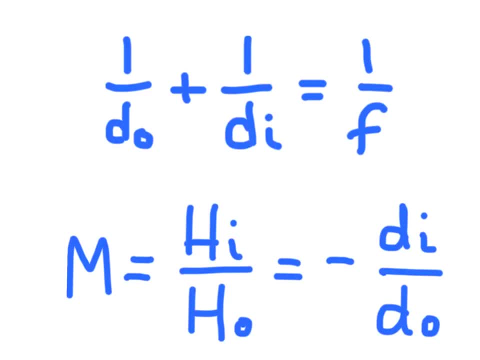 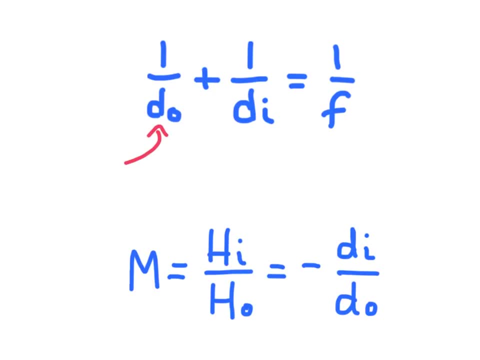 This is called the magnification. This is called the magnification. Now, we really use these equations together when we're solving problems, and I'll tell you what the different variables mean here. So this is the object distance, this one is the image distance. 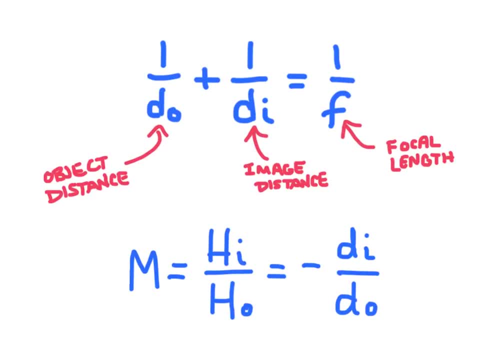 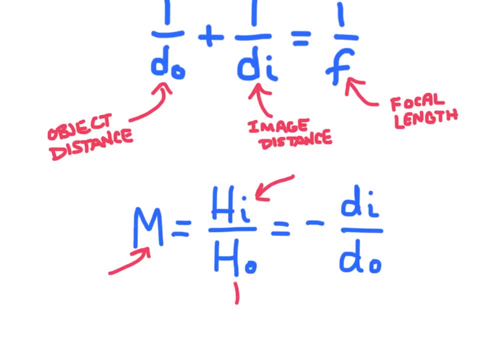 and this one is the focal length of the mirror And then the magnification. right here is a ratio that compares the height of the image to the height of the object, And magnification can be solved two ways. We can use the height of the image and object, or the distance. 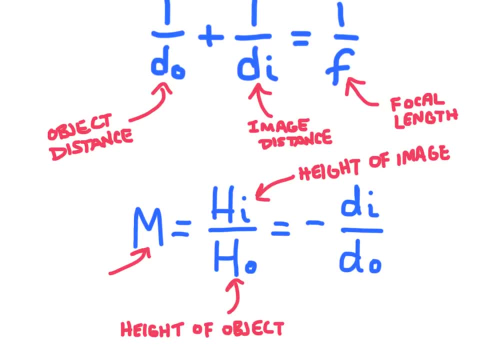 ve bothered to use theулces as ah have detailed hues for, so the object distance or the distance of the الم, substituting the lengths, Simon says, or something haveressea than the distance. At least we've worked on this already at the climate app. 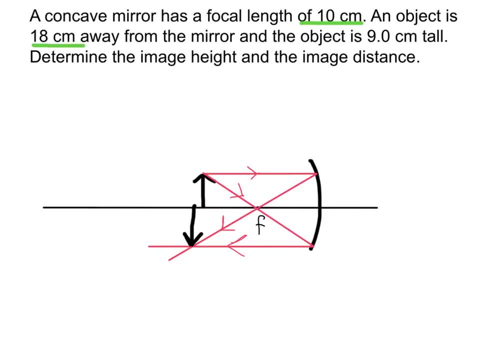 In the Smart software within this device, there are common methods for calculating the lengths and distances of objects that are ilauped, ranging from le 진چ, By distinguish the size and length of the object versus the distance of theー image, and distance of the object. 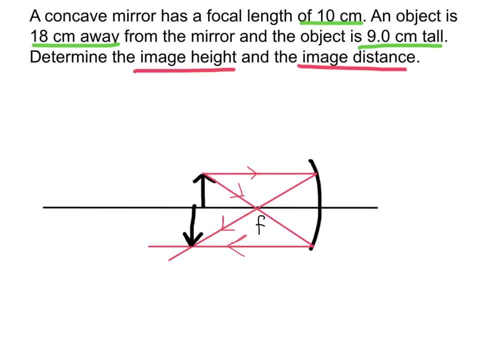 So let's try using these equations to solve a problem. So this says that concave mirror has a focal length of 10 centimeters and an object is 18 centimeters away from the mirror: the object which is right here, and then the image that is produced. 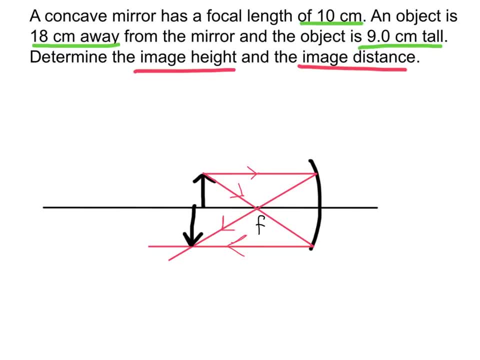 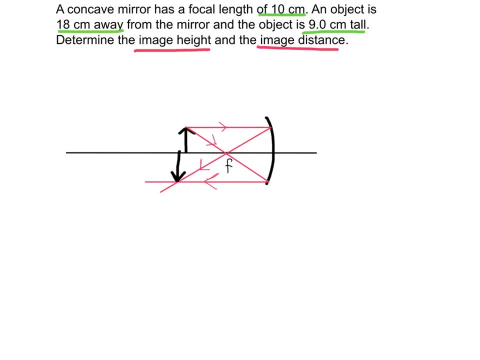 And we're going to use the magnification equation and the mirror equation to determine the height and the distance. So let's start with the distance. So here's our mirror equation and we're going to solve for the image distance. and that's this guy right here. 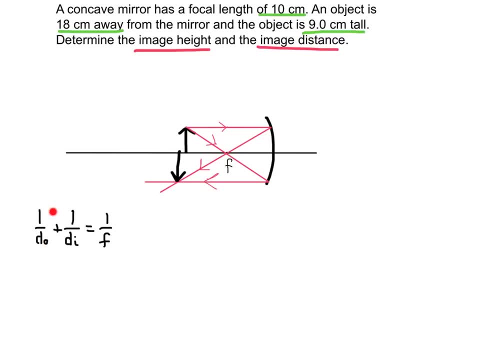 So I'm going to subtract 1 over DO from both sides, so it's going to get rid of it here, it's going to move it over to this side, and so I end up with this, And now I'm just going to go. 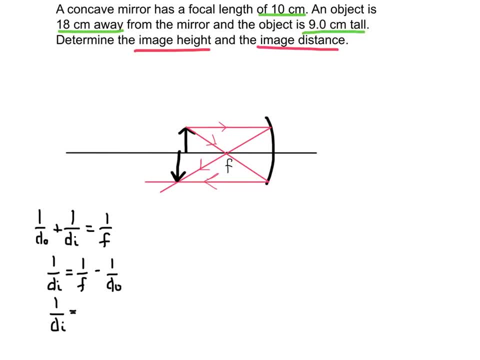 ahead and plug in the numbers here. So I have 1 over the focal length of 10 centimeters and 1 over the object distance of 18 centimeters. that's right up here. Now I can literally just plug into my calculator if I want 1 divided by 10, and then subtract that one from 1 divided by 18,. 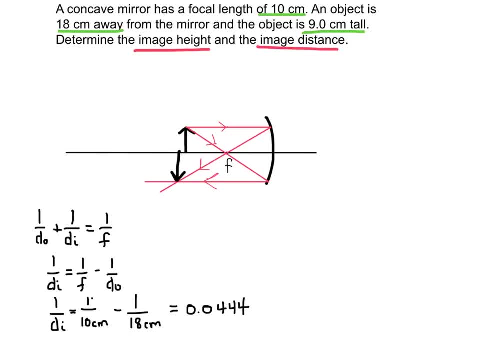 and I would end up with 0.0444.. And this is representing 1 over the image distance. So I would just need to take the inverse of this number right here, or just take 1 divided by that number, and I'm going to get.